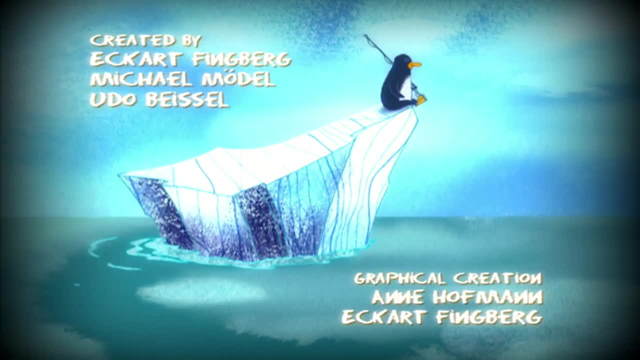 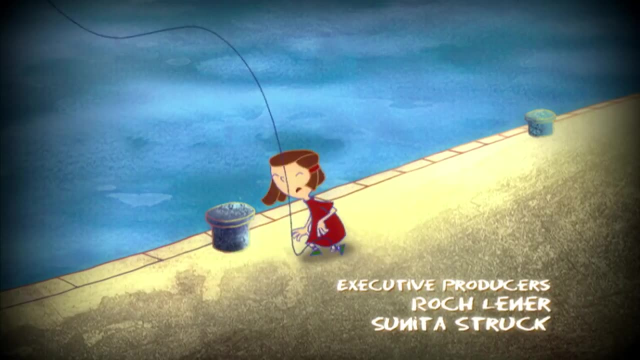 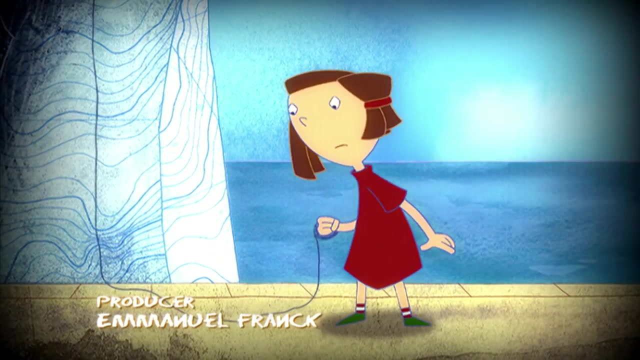 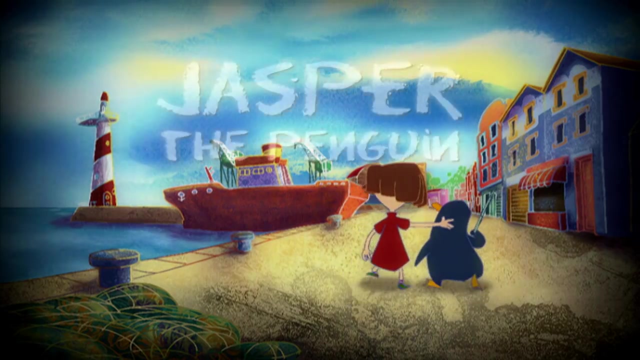 Ahoy, Ahoy, Ahoy. This is Jasper With a letter from way over the sea. Ahoy, This is Jasper With a tale of my friend Emma and me. So, on the shore, keep a lookout for a message in a bottle on its way from yore. Jasper. 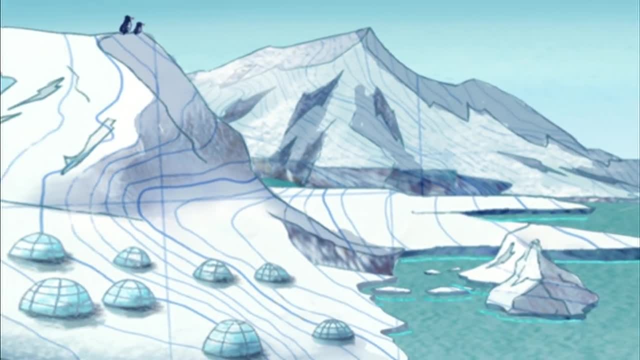 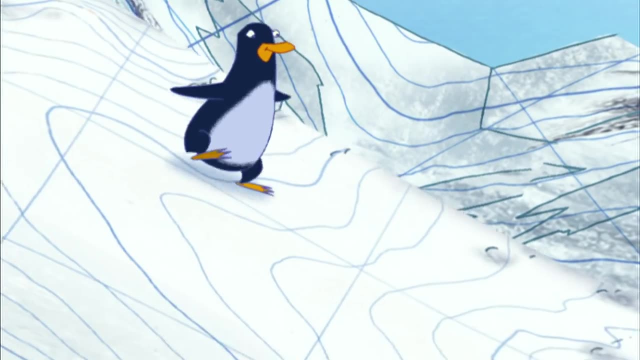 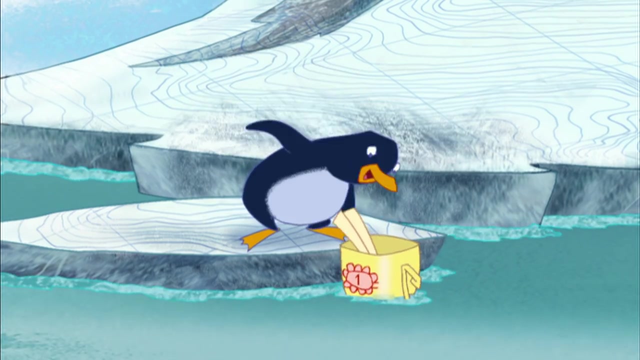 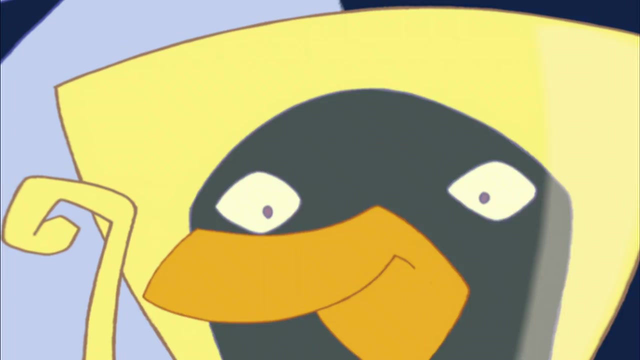 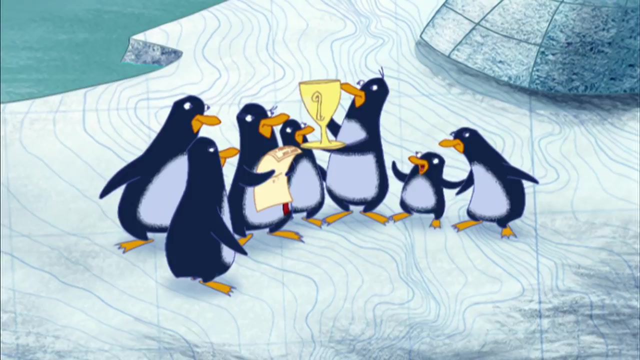 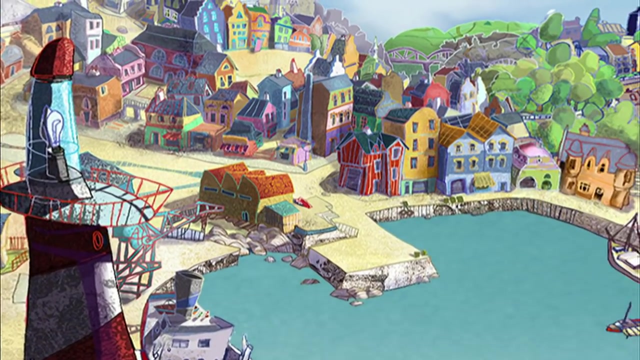 Ahoy from the other side of the world. What you see here is a winner. I received it because I lost a stick I should have been taking care of Huh. It all began because Emma had to go to the sports competition today And, of course, 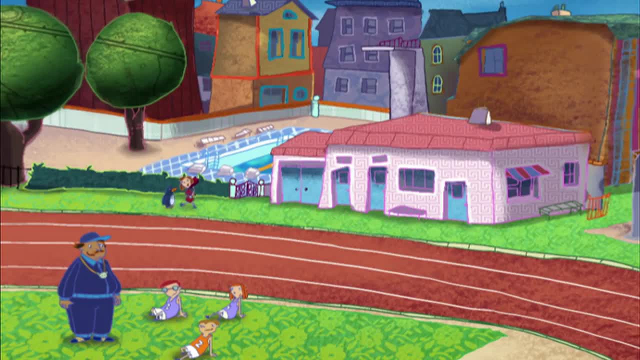 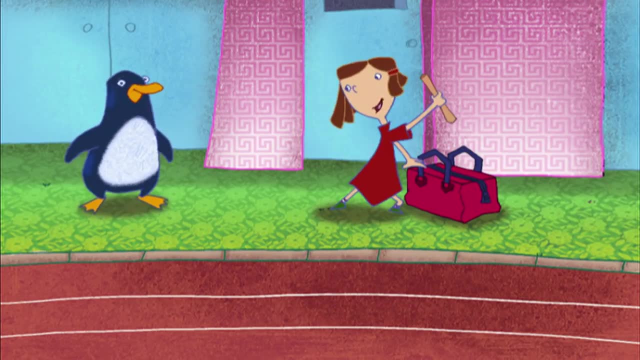 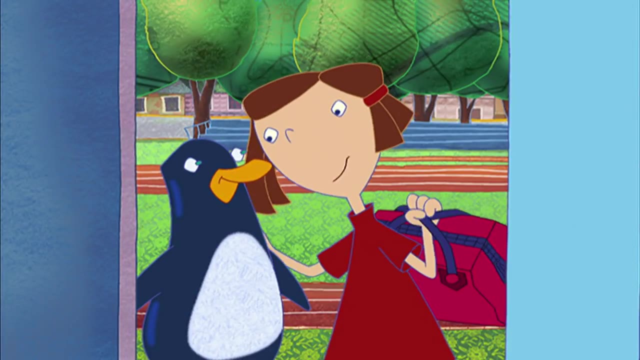 I went along too. This is a relay race baton. There are four people on each team. One runs with the baton and to the next who runs till he reaches the winning post. One from the left comes from the left and the other from the right. 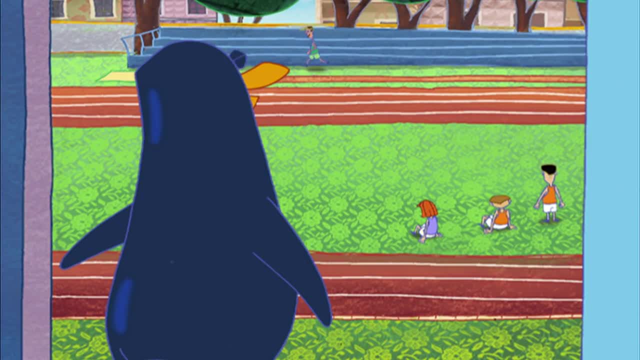 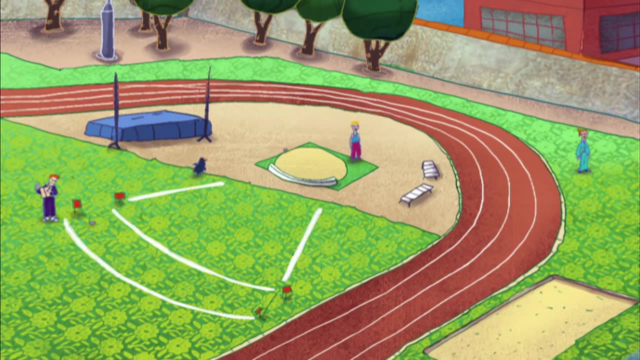 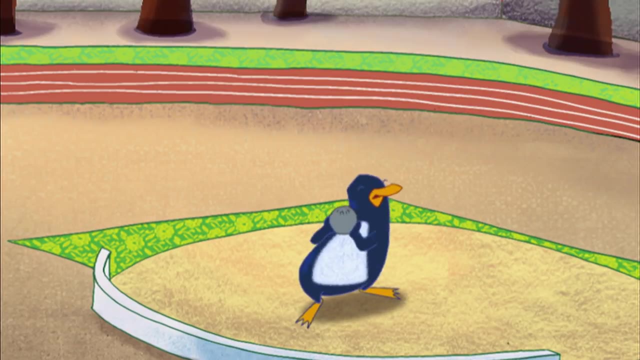 Two from both teams run into the wall and reach the ball. Last but not least, empty the playise and the puzzle box. atten palate again. They need to eden each other to find another hat to lean on, And that's it. 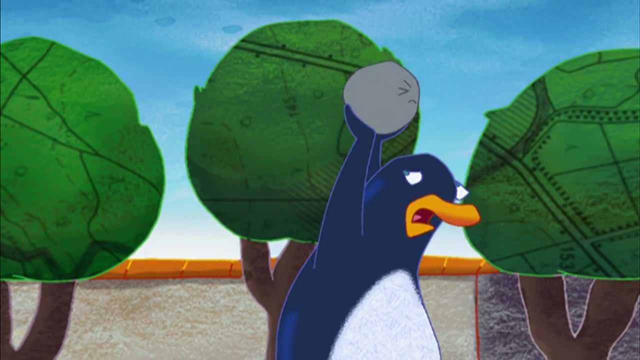 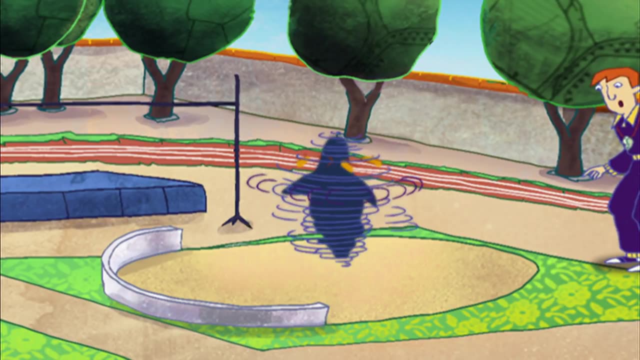 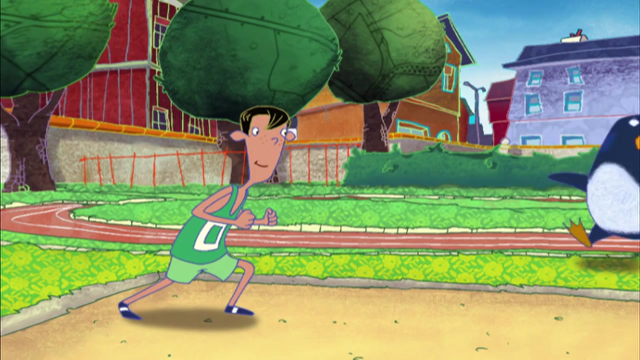 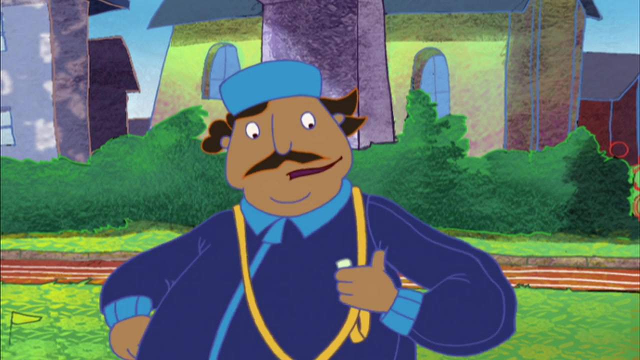 I'll need that Princess to pet my little baby, little dog, And all the wimpies should go to Ka brain thingy. Great, Welcome back, Grah. That was the best result so far. All right, the next jumper please. 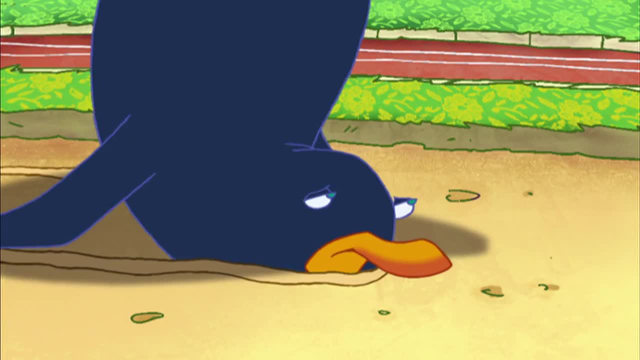 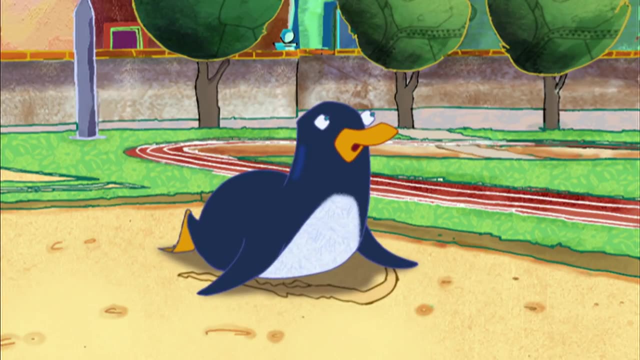 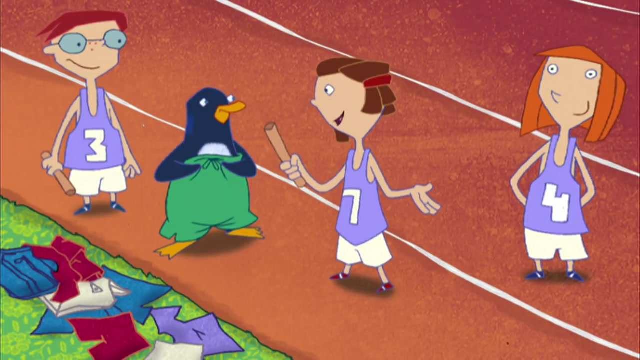 Ah, Lucky that you're here, Jasper. Ah, Michelle has got a cold and can't come. You have to run, for our team Will do. OK, I come running and give you the baton, You take it and run to the finishing line. 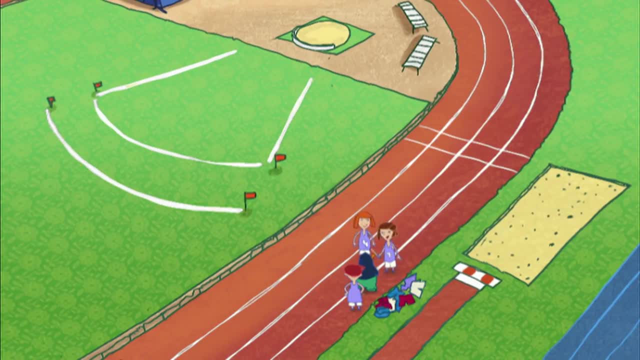 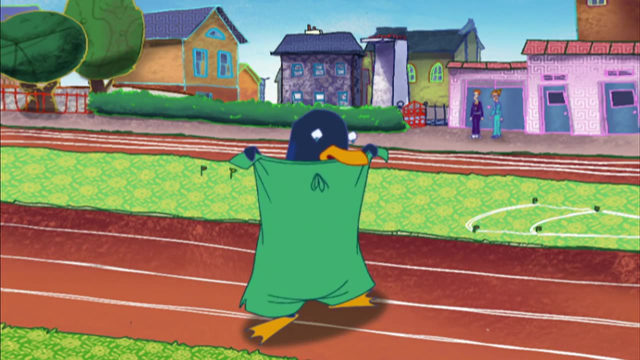 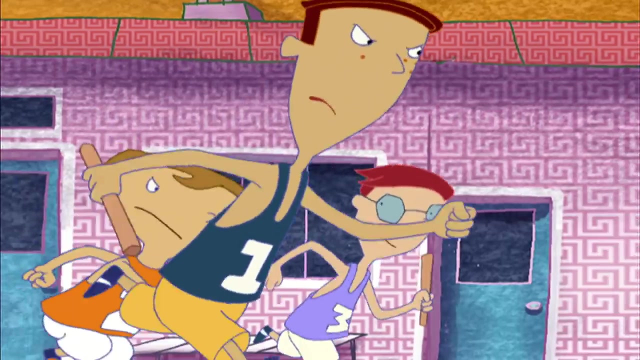 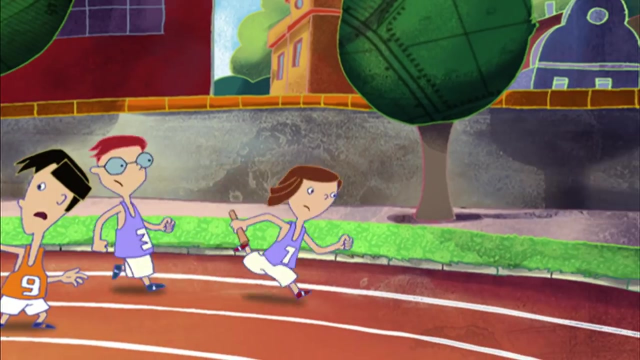 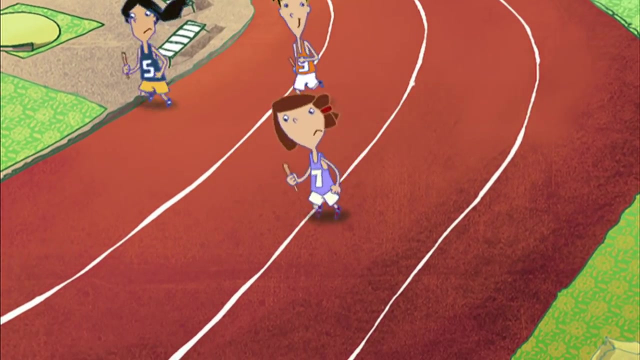 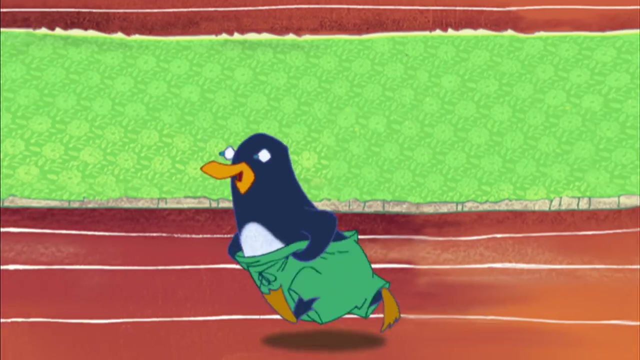 Only, you can't lose the baton. Whoever loses it loses the race. See you soon, OK, bye, Oh, Ready, WHISTLE, BLOWS. Start running, Jasper. I'm almost there. Run, Jasper, run. 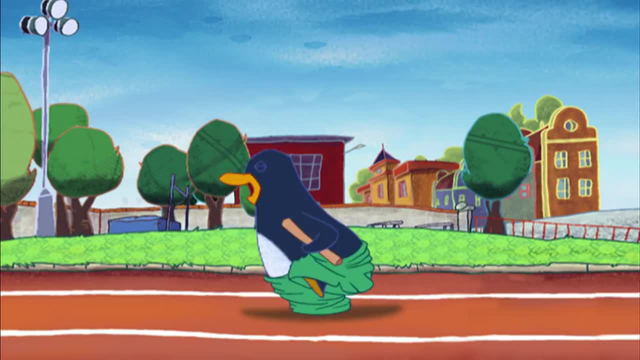 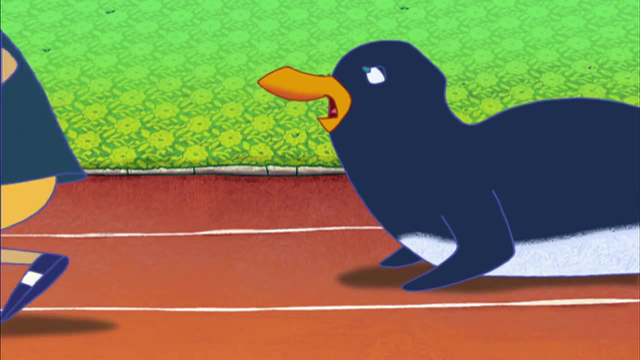 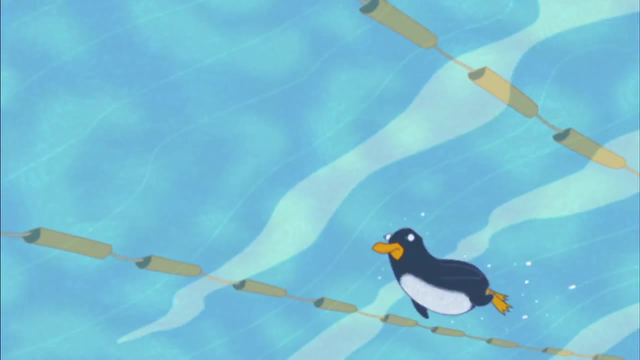 WHISTLE BLOWS, WHISTLE BLOWS, WHISTLE BLOWS. Oh no, The baton. I have to get it back. Hands off, That's Emma's baton. WHISTLE BLOWS, WHISTLE BLOWS. 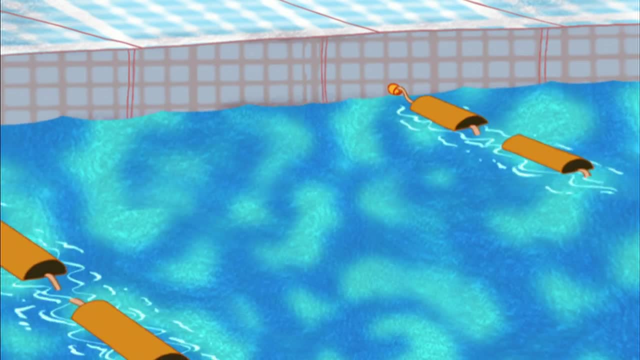 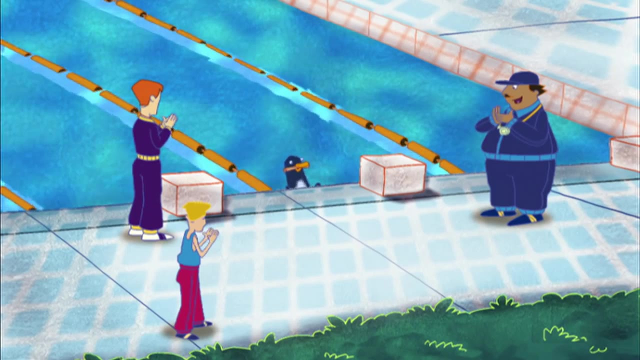 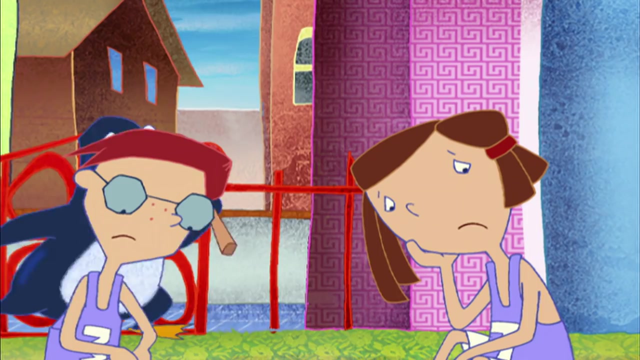 WHISTLE BLOWS, Great WHISTLE BLOWS, WHISTLE BLOWS, OOF adults laugh, 談他话. CHESTNUT CRYING, CHESTNUT CRYING. It bounced off. I tried, I had, I did. 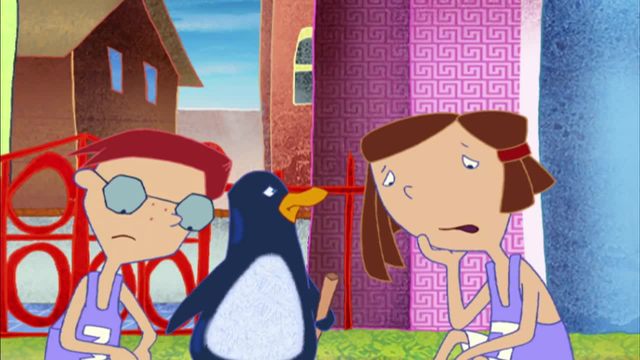 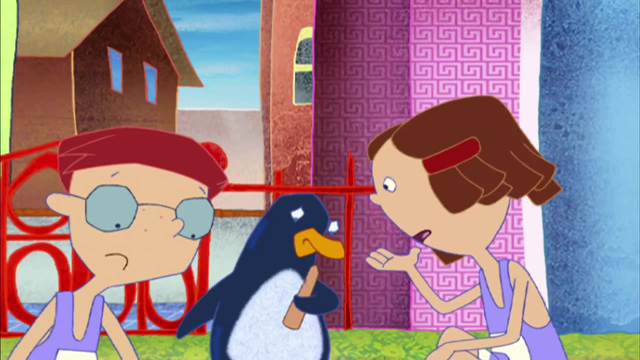 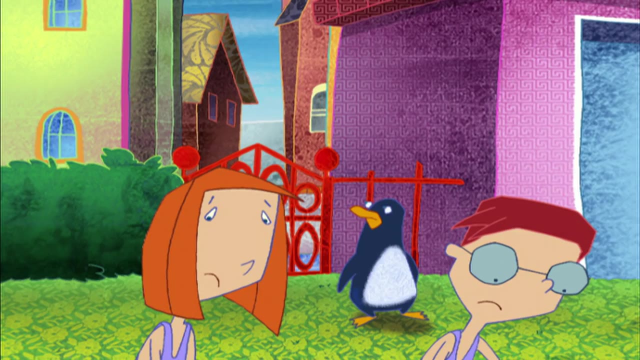 Oh well, here's the baton. We lost the race, didn't we? We lost the race. Don't feel bad, Jasper, Your shorts were just too big. Hey you, I've been looking for you everywhere. You were just in the pool, right. 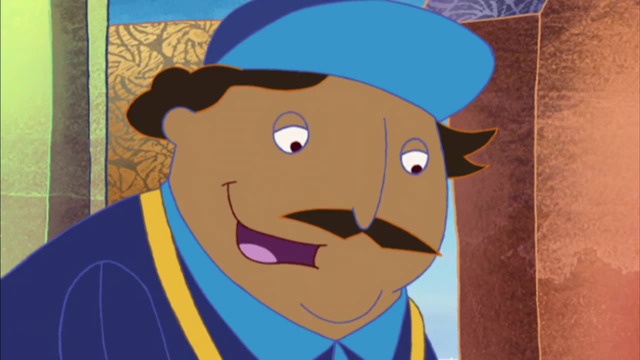 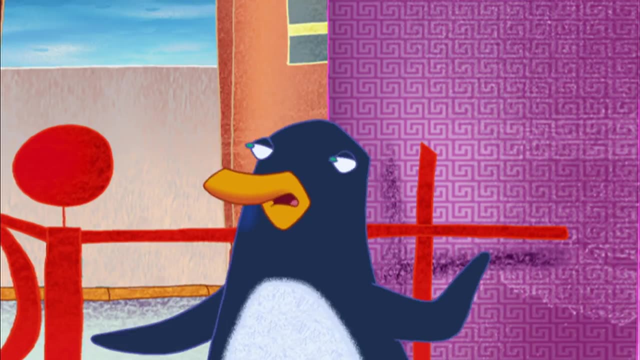 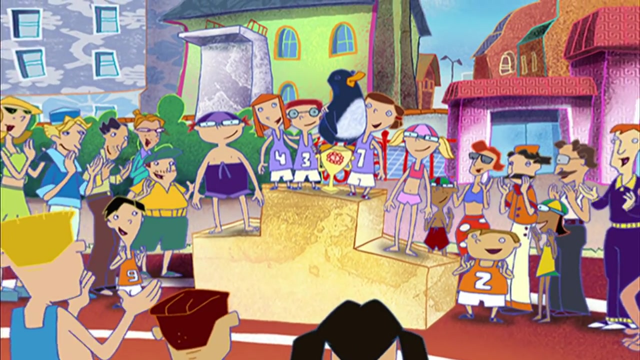 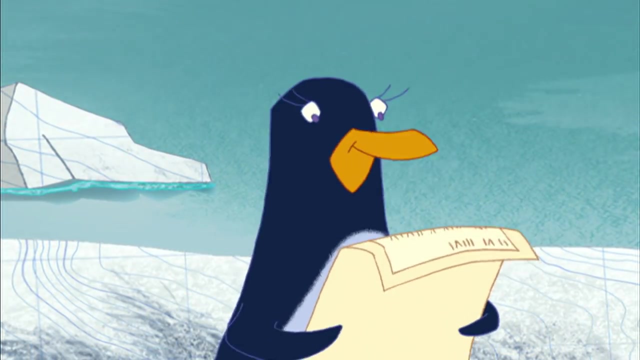 Yes, Then this is your cup. You won it in the swimming competition. Congratulations. But those should be up there too, Them Why They help me work up enough speed. I wish you all a relaxing day without too much running around, And I'll be back soon, But only when I've seen everything.